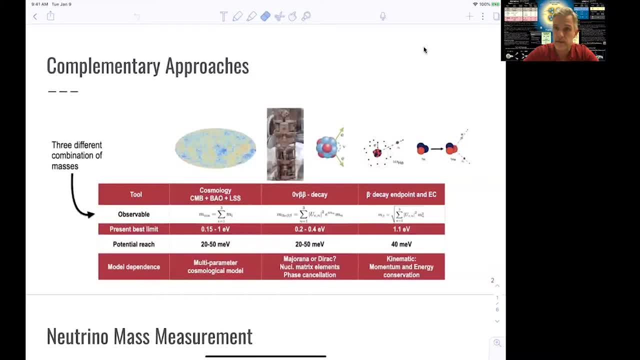 the question whether or not the a neutrino is a Dirac particle or a Majorana particle, as we discussed in earlier lectures. And then there is the more classical approach of measuring the mass of a neutrino from the endpoint spectrum of beta decays. 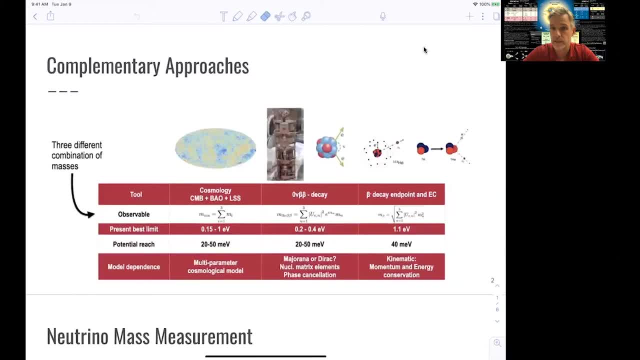 And so here, the current best limit is from the Katrin experiment- And I'll talk about this on the next slide- And it's in the order of 1 electron volt, And there's a potential reach to go down to 40 milli-electron. 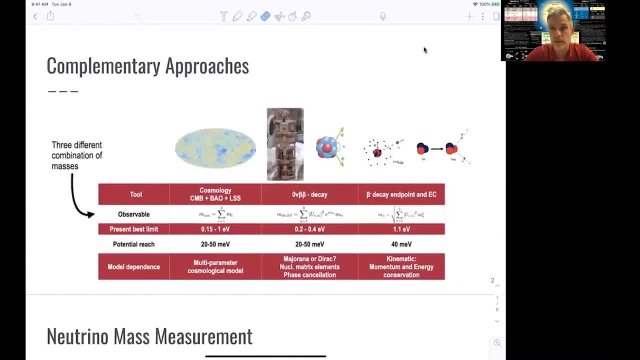 volt. So currently the range of limits is in the order of 1 electron volt, so a bit better, And one will be able to go down to limits in the order of 20 to 50 milli-electron volts. So here is a cartoon of how those measurements are. 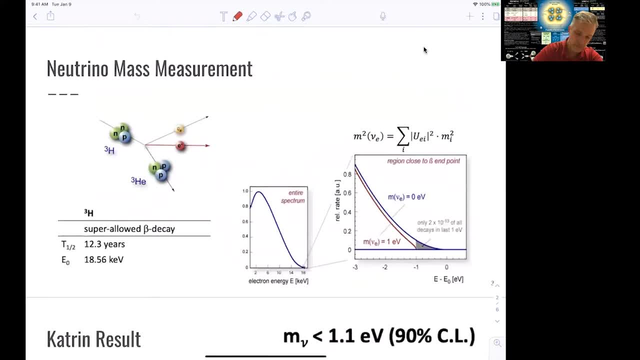 being conducted. One starts with tritium and uses beta decay, And this lecture overall is a good kind of first entry into the nuclear physics program where we discuss beta decays and other nuclear decays in more detail. What we find here is that we find an electron. 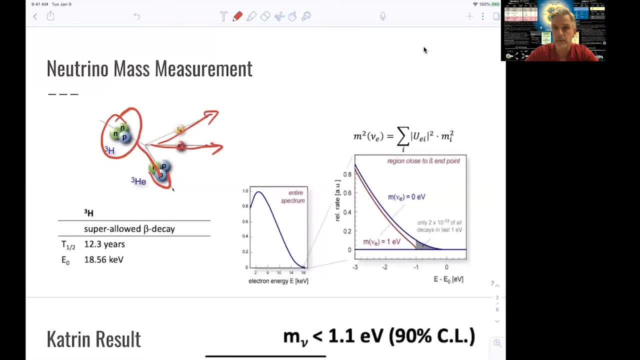 and then neutrino- antineutrino in this case- being emitted, And so the name of the game is now to measure the electron energy as precisely as possible and then find a sensitivity of the neutrino mass in the endpoint spectrum And those small differences here in the endpoint spectrum. 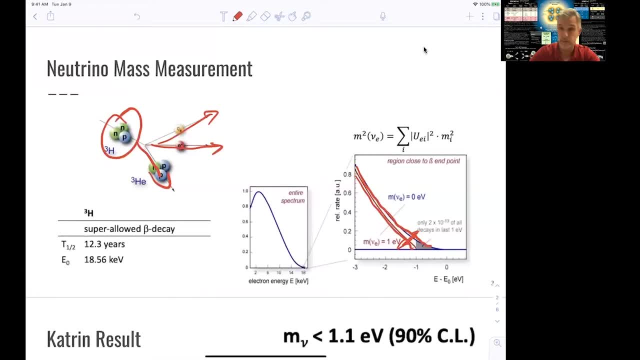 they then lead to understanding of the mass of the neutrino, because the total energy in the collision needs to be preserved, And so the entire story here is about how precisely can we measure the energy of the electron in order to infer the neutrino mass in that. 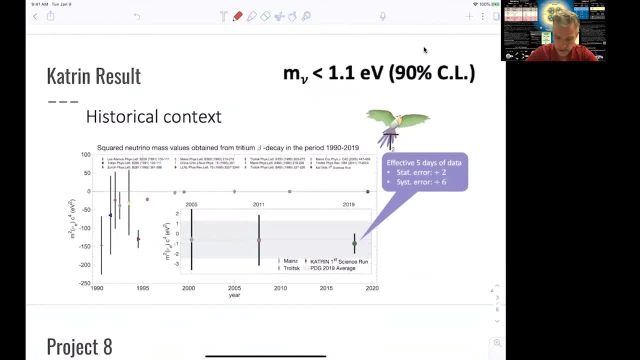 And so the latest results came out. The results came out last year from the Katrin experiment and shows that we can set an upper limit- The result is consistent with the neutrino mass of 0- and that we can set an upper limit at 90% confidence level. 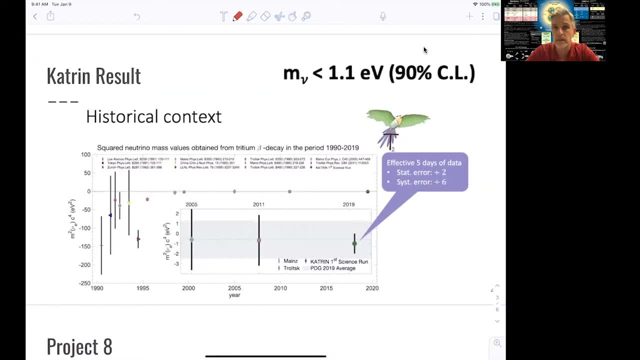 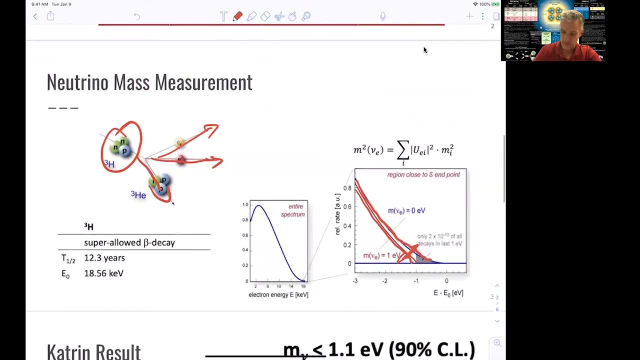 that the neutrino, the electron neutrino, is of mass of 1.1 electron volt. Just as a reminder, we measure the mass of the electron neutrino in this decay, which is the sum of the individual components: mass eigenstate. 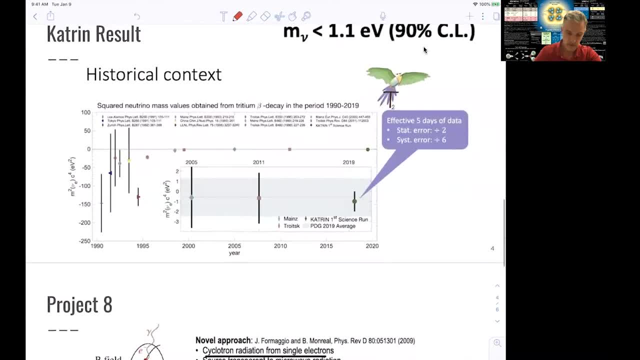 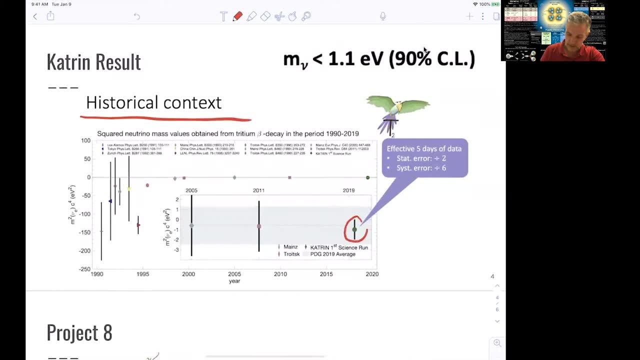 which make up the electron neutrino. To set the historical context in this discussion here, we find that this latest result is an improvement of the order of factor of 2 compared to previous results by other experiments which had a very similar job to measure the electron energy. 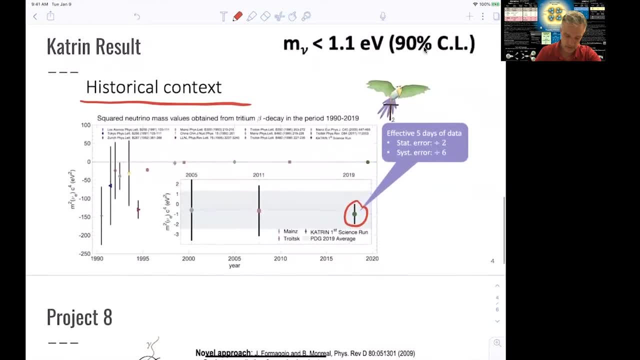 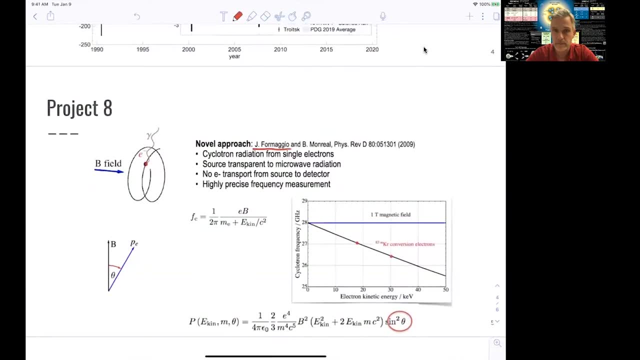 in beta decay. In the end point spectrum of beta decay There's a new approach which has been proposed by Joe Formaggio here from MIT, which changes the way the electron energy is being measured. So the idea is to have the decay happen in magnetic fields. 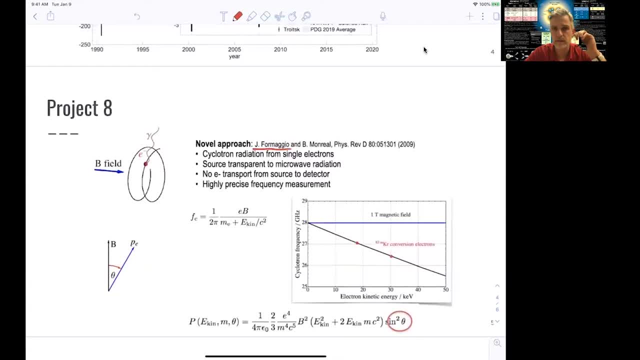 and use the cyclodon radiation of single electrons. So the advantage here is that one doesn't have to move the electron somehow. One can move the electron somehow into a spectrometer but can immediately measure the energy of the electron And the measurement of the energy. 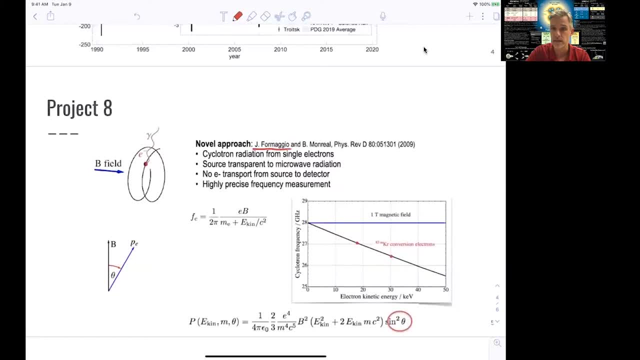 then turns into a measurement of the frequency and basically measures the cyclodon frequency of the electron circling around in a magnetic field. And so it turns out that one moves the measurement of the energy of the electron into a measurement of a frequency, And this can be measured with very, very high precision. 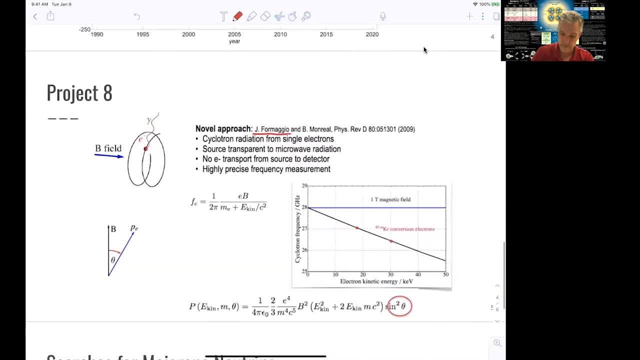 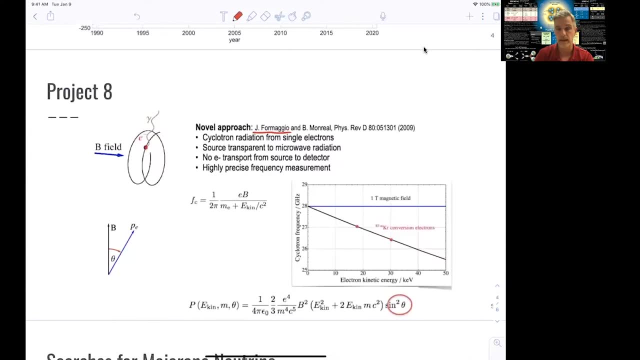 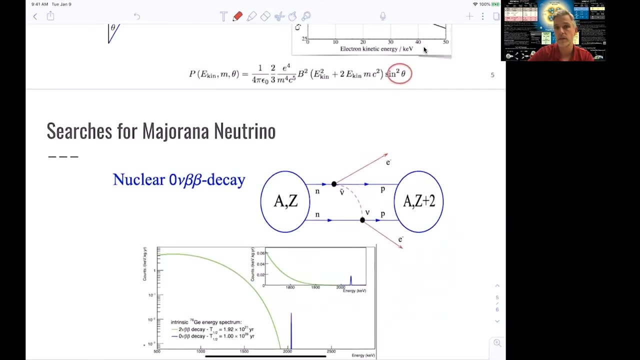 But there is some hope that this kind of measurement leads to very, very precise results of the energy of the electron and with that the mass of the neutrino. So the last slide here is now: how can we figure out whether or not the neutrino has Dirac or Majorana nature? 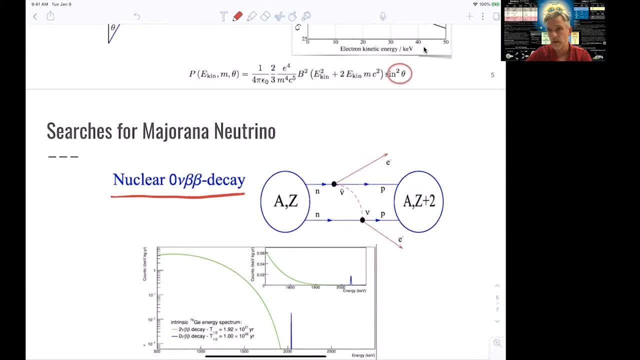 And this can be done- or the highest sensitivity comes from so-called neutrino-less double beta decays. So one starts with nuclear decays where two electrons are emitted but no neutrino, And so this requires that in this process 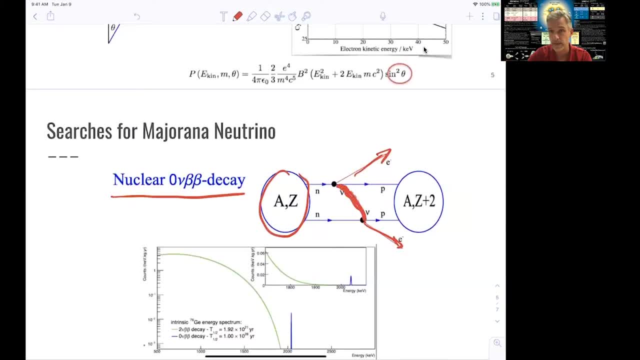 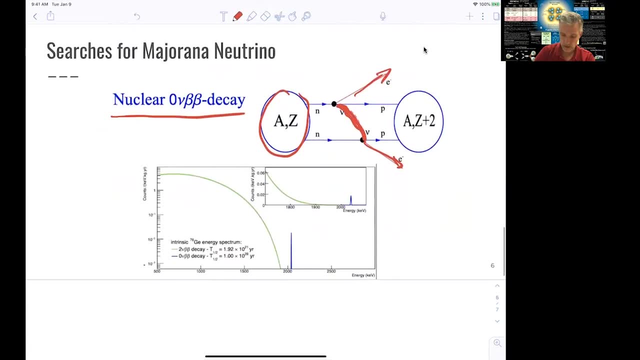 there is a transition which includes the neutrino, where the neutrino has to be its own antiparticle And that just means that the neutrino is of Majorana nature. This is being done by measuring again the energy spectrum And you typically have background all kinds. 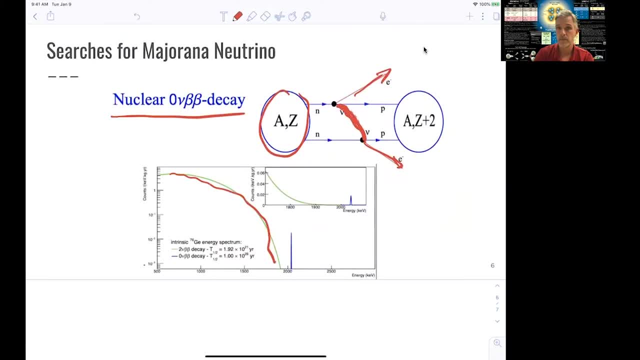 of background contributions, but also backgrounds from double beta decays with two neutrinos. So you see the spectrum here And then you look at the endpoint of this part here and find that there is this peak, a very precise, sharp peak of the energies of the two electrons. 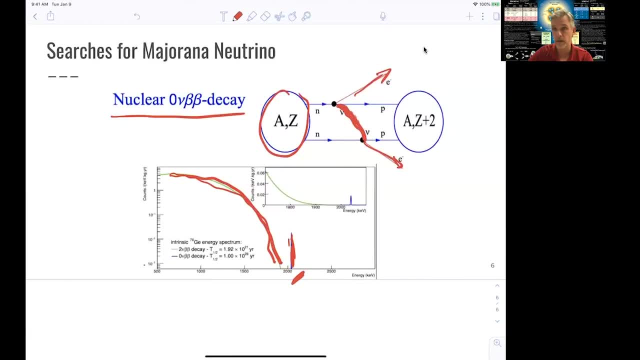 The issue is that forecasting where this peak is requires proper knowledge of the dynamics inside the nuclei. here, And those measurements are being conducted. There's many of them conducted in various nuclear transitions or decays And they haven't yielded a positive result yet. 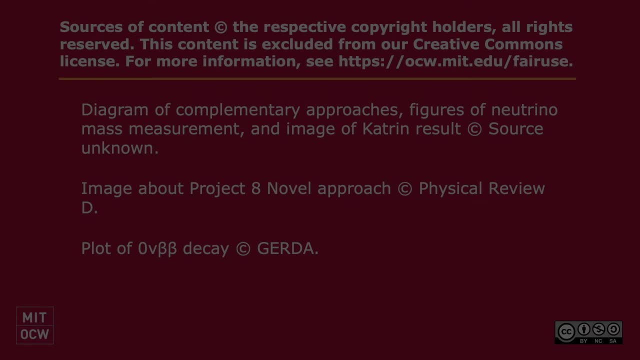 Research is still going on on this end. 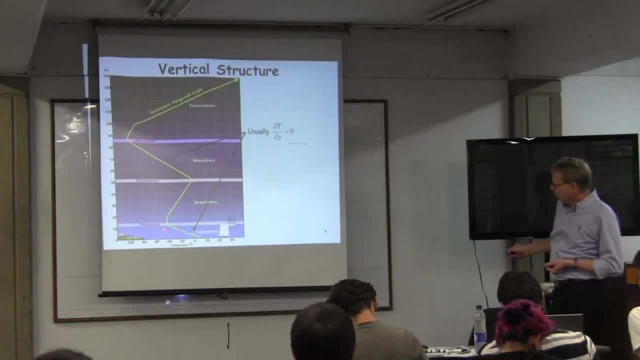 So the temperature drops rapidly. I think we even reached 50 minus, that's what the computer said. But then there is a tropical pause- generally these pauses here- where the temperature does not change with altitude, And then this trend or the gradient is reversed, And then it actually gets slightly warmer when you go further up. And it goes into the mesosphere, gets a lot colder again and then it increases. So these layers are then called the inversion layers, where the temperature gradient changes. Since it's inverse gradient, it's an inversion layer, And this is essentially the same, just a bit more what we expect at those heights. 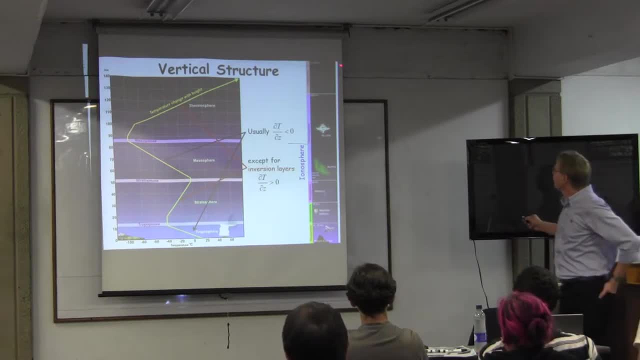 This goes up to 10,000 kilometers up here, So this is not to scale a person. this is 630 kilometers, But you have the mountains here and the airplanes that can fly up to whatever 15 or maybe 20 kilometers. 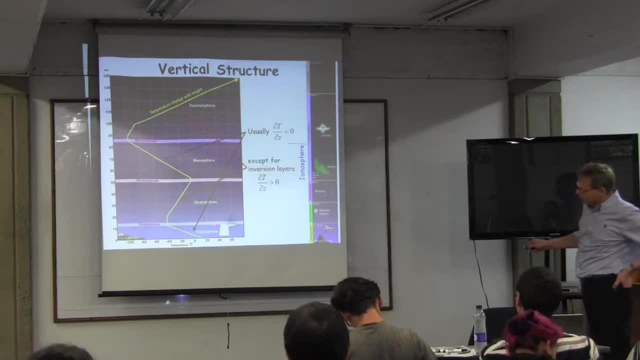 If you want to get above this atmosphere- and there is a reason for it, because that's also the height where the clouds can be set up- If you go above that, then you need- or you want to go above that, you need- some weather balloons.